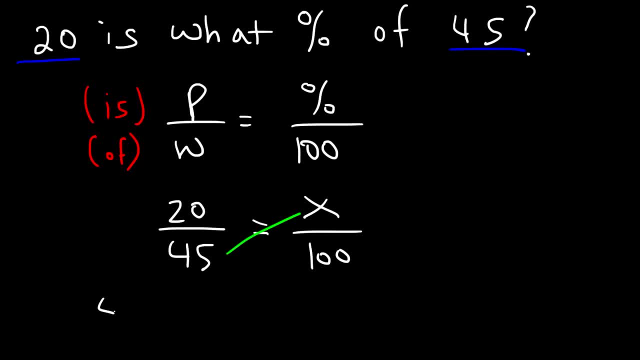 let's multiply 45 times X is simply 45 X, and then we have 20 times 100, which I'm going to leave it like this: now 45. let's divide both sides by 45, so X is going to be 20 times 100, which is 2000. 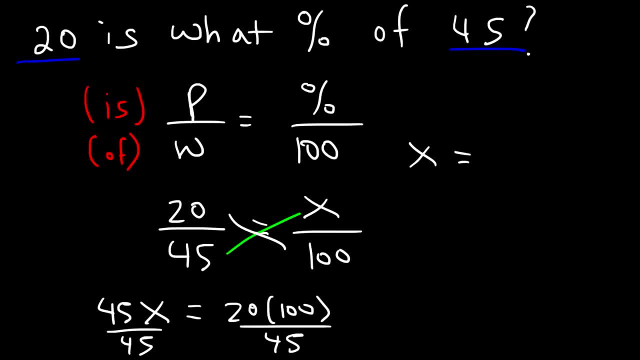 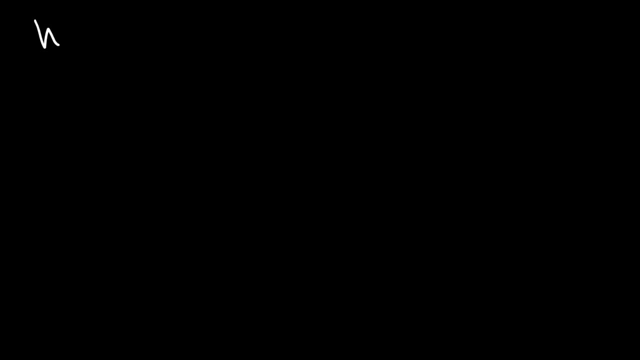 and 2000 divided by 45 is about 44.4. so that's the answer: 20 is 44.4 percent of 45. here's another similar example: what percent of 12 is 27? feel free to try that problem. so we're going to use this example. 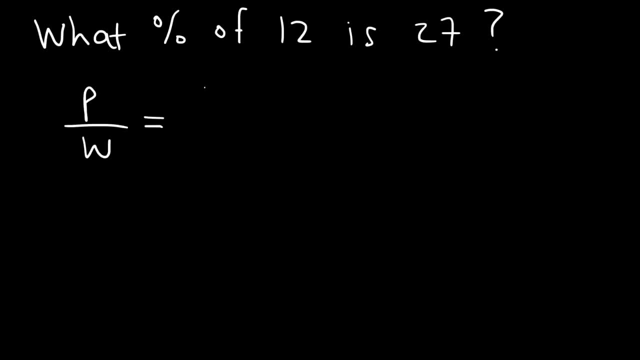 same equation. part divided by whole is equal to percent divided by 100, the percent we're going to make it X. now what is the part and what is the whole in this problem? the number that is associated with is is the part, so 27 is the part. 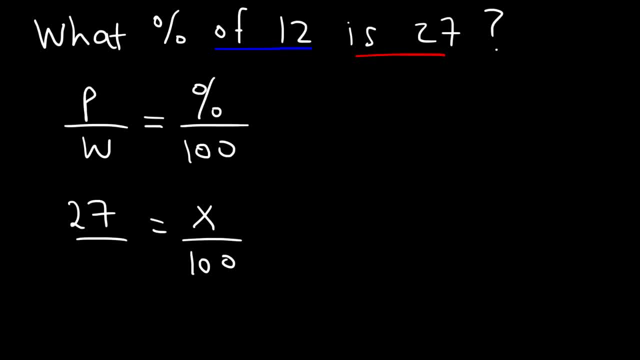 the number that is associated with the word of is the whole, so 12 is the whole. so what percent of 12 is 27? whenever the part exceeds the whole, your percentage is going to be greater than 100. let's go ahead and find the value of X. so what we have is 12 X after cross. 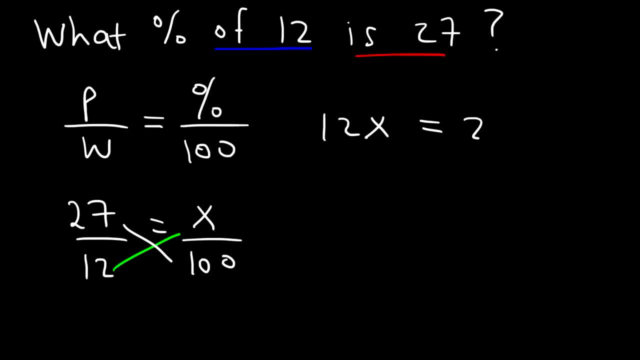 multiplying is equal to 27 times 100, which is 2700. now we need to do is divide both sides by 12, and then this is going to give us the answer. so 2700 divided by 12 is 225. so 12. well, 27 is 225 percent of 12, and so that's how you. 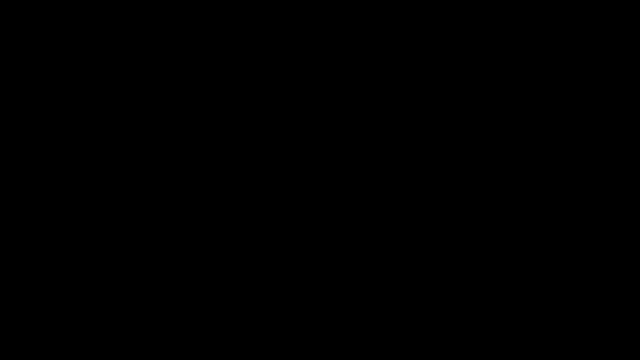 could be the sentence if you want to, but that's the answer. now. the second thing that we need to talk about is how to find the part. this question is going to illustrate what is 32% of 86, so let's write the equation. first, we have the. 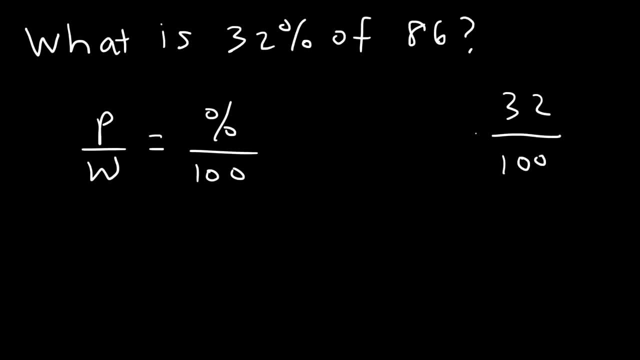 percentage: 32%. now the number that's associated with the word of is 86 and that's the whole. so we're looking for the part which we can replace it with X, and now we just got across: multiply, so X times 100 is 100, X, and 86 times 32. 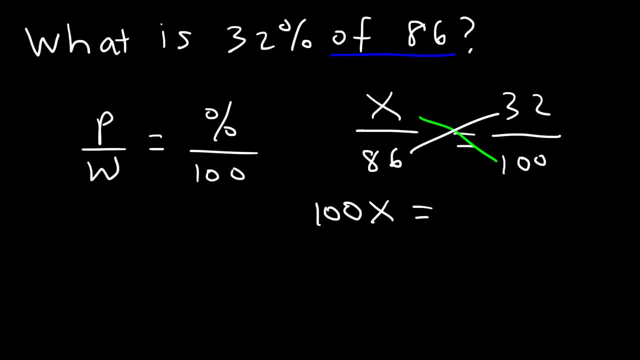 find the value for that. that's going to be 27, 52. so we got to do is divide 2752 by a hundred, and that's equal to 27.52. so 27.52 is 32 percent of 86, and that's the answer. here's another example: what number is 21% of 250? 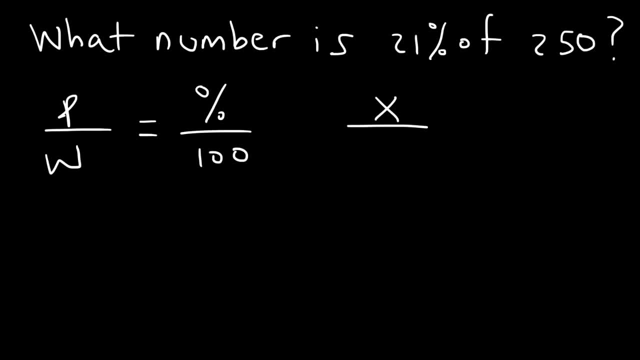 so we're looking for the part. once again. let's replace P with X. the whole is the number associated with the word of. that's 250. we have the percentage, which is 21 percent, and let's cross, multiply. so once again we're going to have a hundred. X is equal to 250 times 21. 250 times 21 is 52, 50. now let's divide. 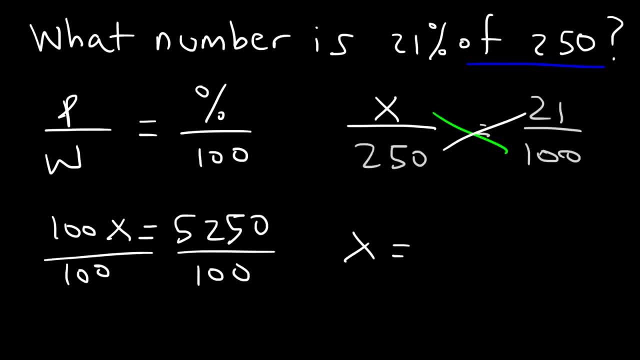 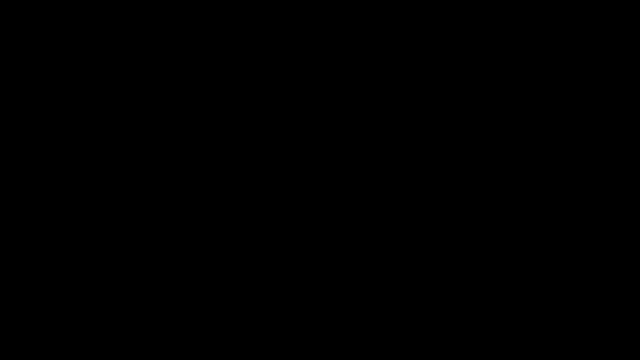 both sides by a hundred: 52, 50 divided by 100 is 52.5, so 52.5 is 21% of 250. by the way, 50 is 20%, 250, 20% is one-fifth. the last thing that we need to cover is finding the base, so here's a problem that will. 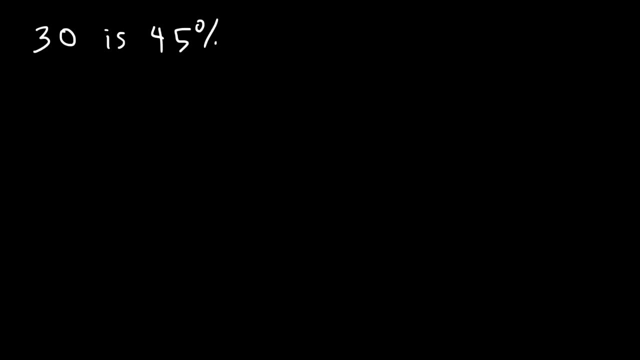 illustrate this example. 30 is 45%. of what number? so go ahead and pause the video and you can try this if you want to. so let's start with the equation: part divided by whole is equal to the percentage divided by a hundred. so in this problem, what is the part and what is the whole? 30 is the part. it's 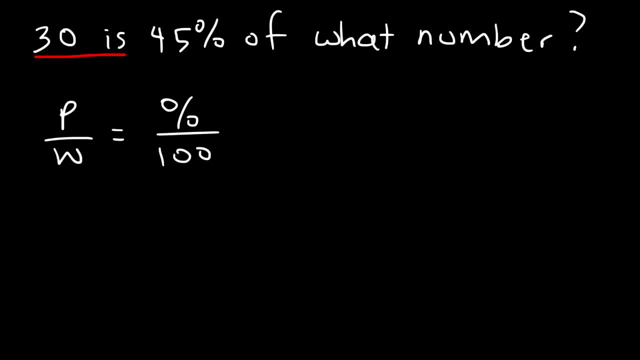 associated with the word is. we're looking for the whole, which is also known as the base. we're looking for the number that's associated with of. so 30 is jusp, the whole or the base is X, the percentage is 45. so let's cross, multiply. 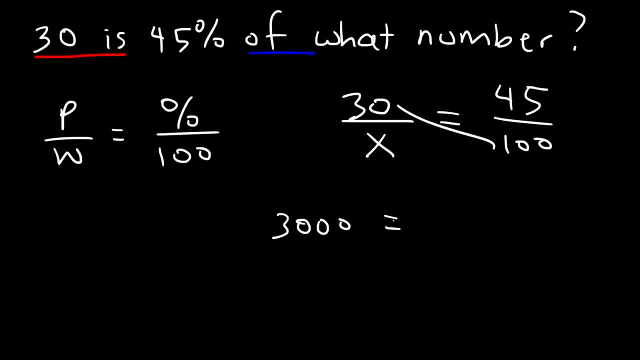 30 times 100 is three thousand x times 45 is 45 X. so let's divide both sides by 45. 3,000 divided by 45 is sixty six point seven. so you can really think of the answer for the common asker. answer for common asker, as long as you start's with: 56.8. so this into x. so it's going to say: and so the %, as we define this as Levlak Nann Anchor that in website we f8 M al 2023: 6. Peter Taifun k與 Мы经оп Janet Republicans finance program for 10th is as interrogating month. So 30 is P, the whole or the base is x. the percentage is 45, 30 times a hundred죠да z street. three thousand X times 45 is 35. So let's cross, multiply 30 times CT. 30 times 100 is 3000X times 46.6, So let's divide both sides by 45. shirt. 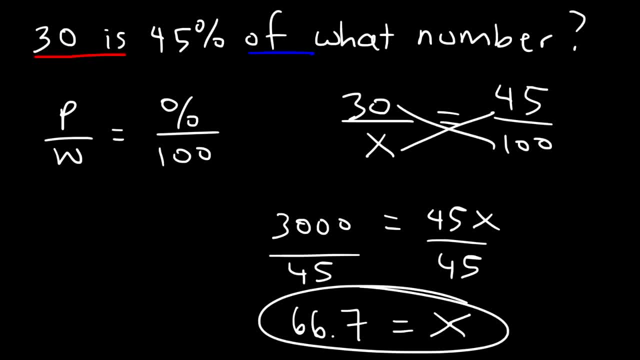 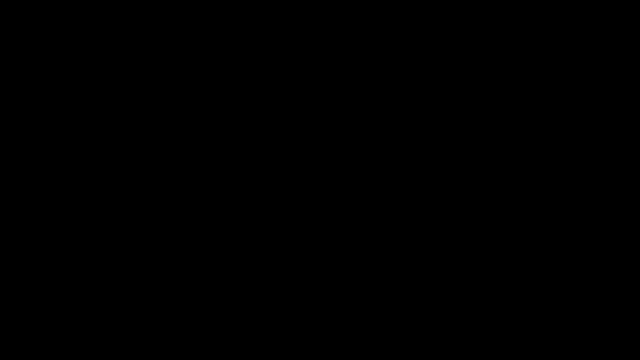 So that's basically the value of x. so that's the base. So 30 is 45% of 66.7.. Here's another example: 34 is 34%. of what number? So in this example we can see that the part is 22 and we have the percentage which is. 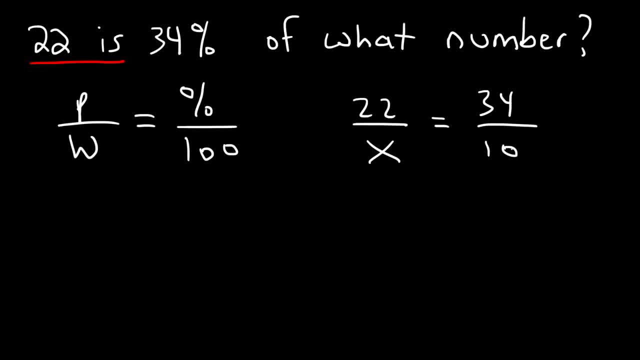 34.. We need to find the whole or the base. 22 times 100 is 2200, and x times 34 is 34x. So let's find the value of x by dividing both sides by 34.. 2200 divided by 34, that's 64.7 if you round it. 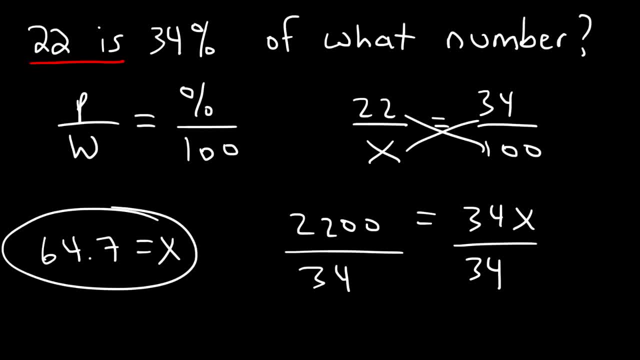 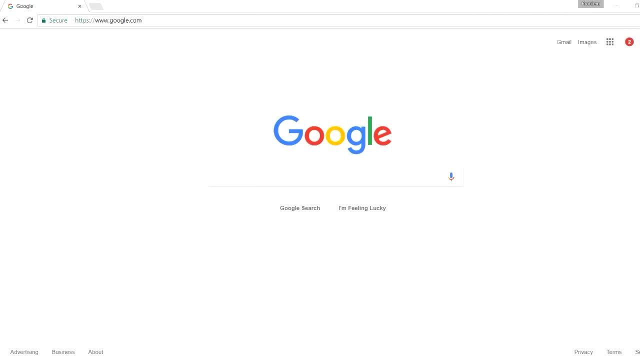 So 22 is 34% of 64.7.. And so now you know how to use the percent proportion formula in order to find the part, the percentage, The percent or the base, which is also known as the whole. Now I want to show you one of my algebra courses that might be useful to you if you ever need. 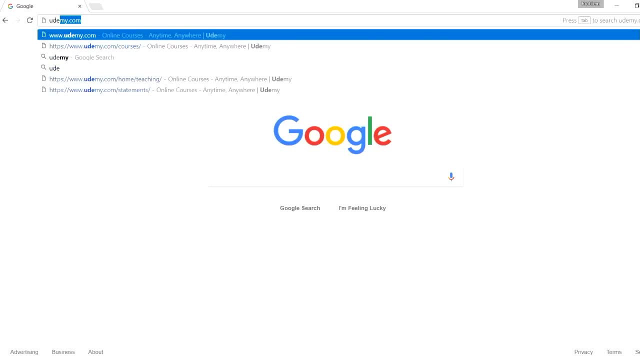 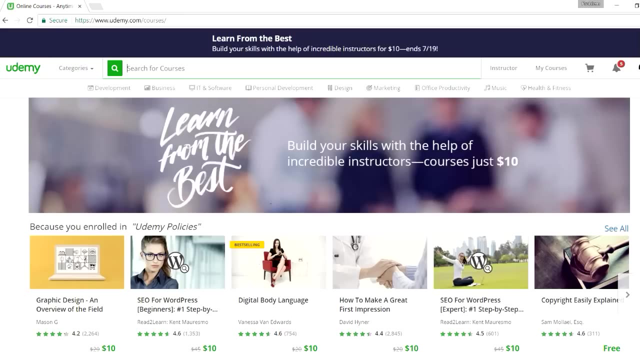 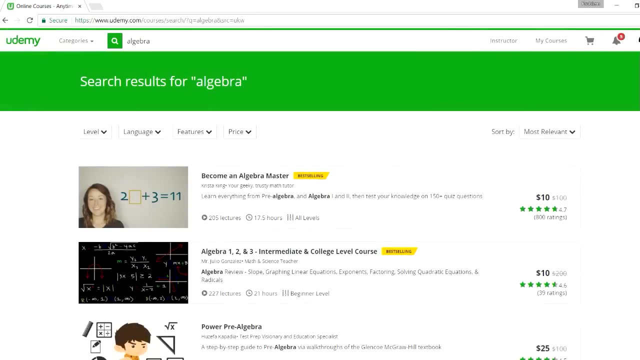 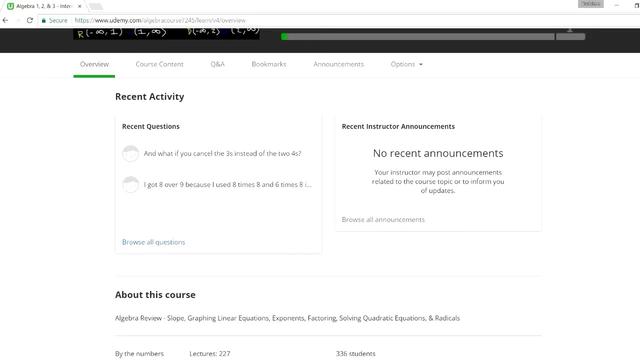 it. So go to udemycom Now. in the search box just type in algebra and it should come up. So it's the one with the image with the Black background. So if you select that option and if you decide to go to course content, you can see what's. 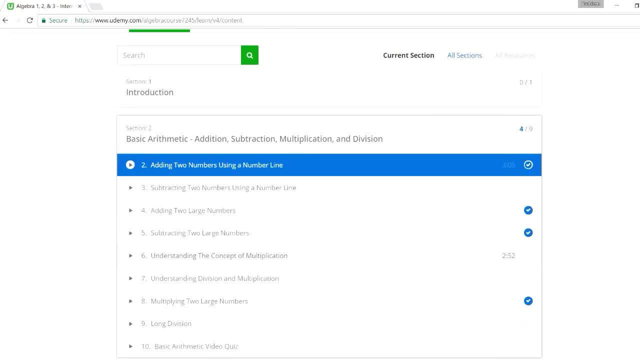 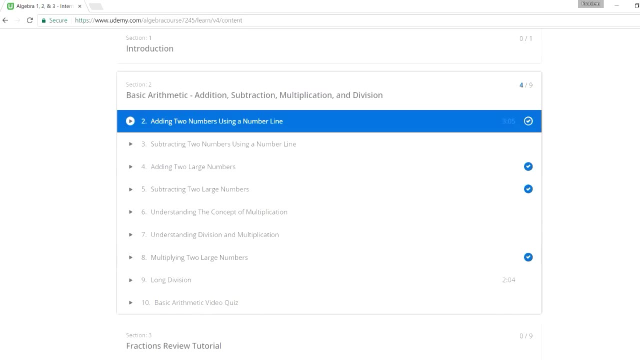 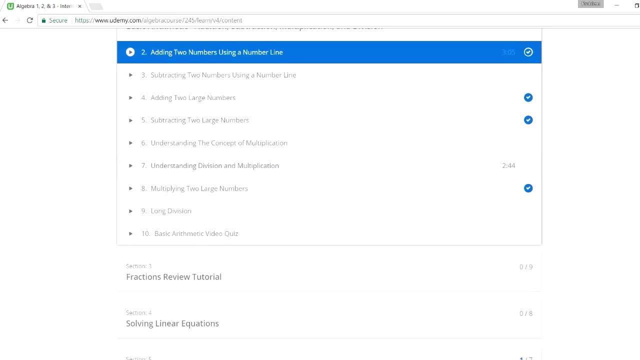 in this particular course. So the first section, basic arithmetic- for those of you who want to focus on addition, subtraction, multiplication and division, And it has a video quiz at the end. It's a multiple choice video quiz. You can pause it, work on the problems and see the solutions. 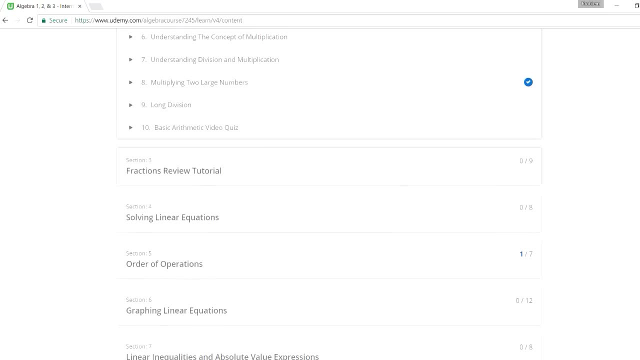 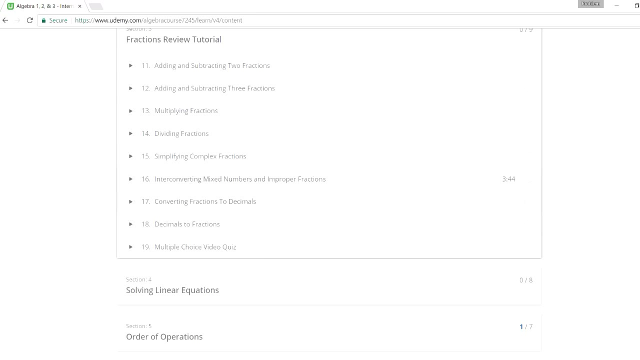 It covers long division, multiplying two large numbers and things like that. The next tutorial is on fractions. Add in subtracting fractions, multiplying and dividing fractions, converting fractions into decimals and so forth, So you can also take a look at that. 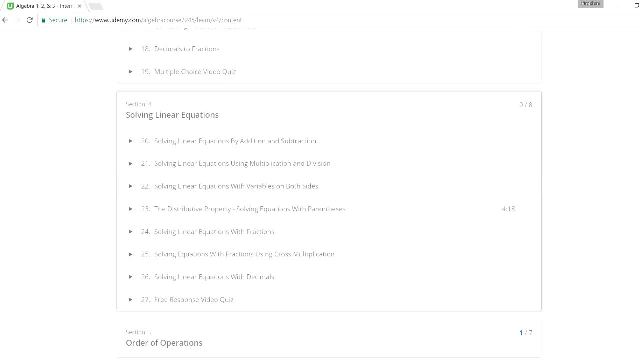 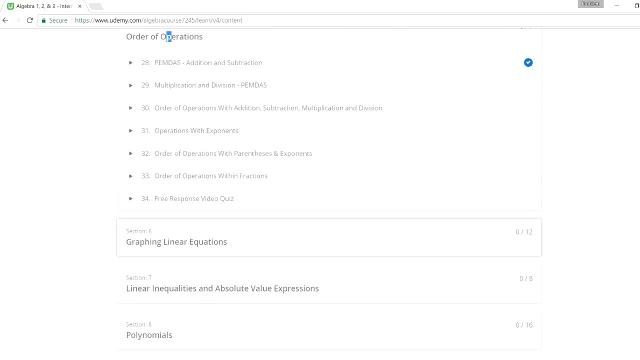 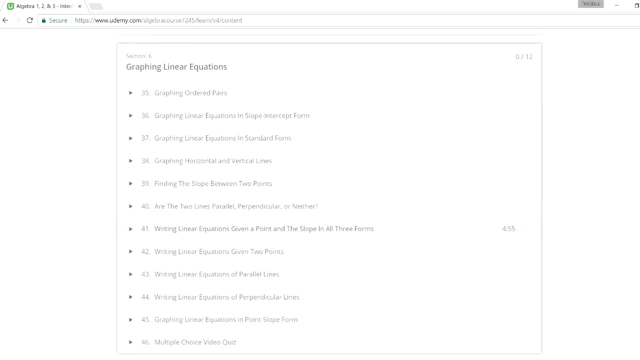 Next, solve the linear equations which we covered, And just more examples if you need more help with that. The next topic, order of operations, Which is also useful Graph in linear equations. You need to know how to calculate the slope. You need to be familiar with the slope. intercept form, standard form. 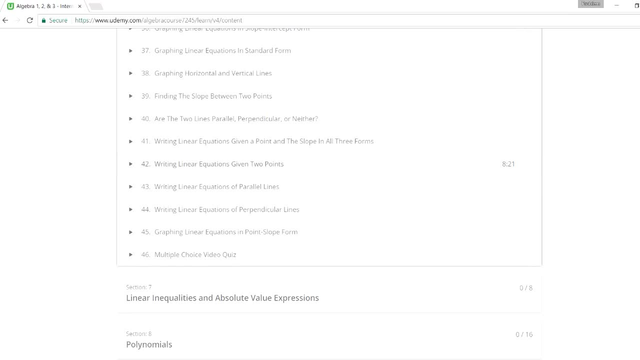 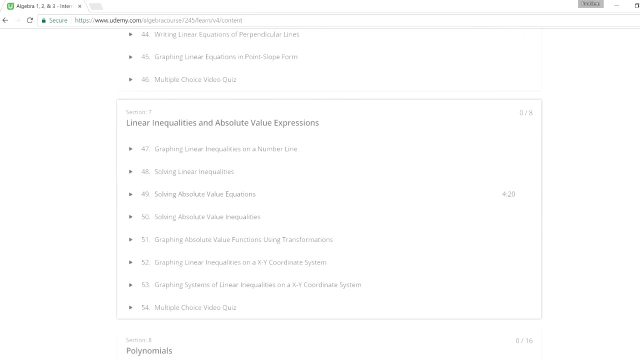 And just how to tell if lines are parallel, perpendicular and so forth, And there's a quiz that goes with that as well. The next topic is on inequalities and absolute value expressions, Which are also seen in a typical algebra course. And then we have polynomials. 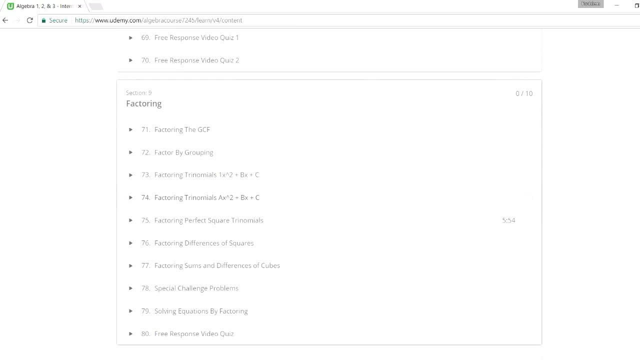 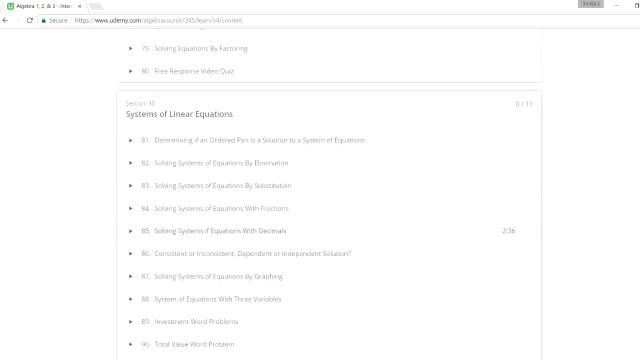 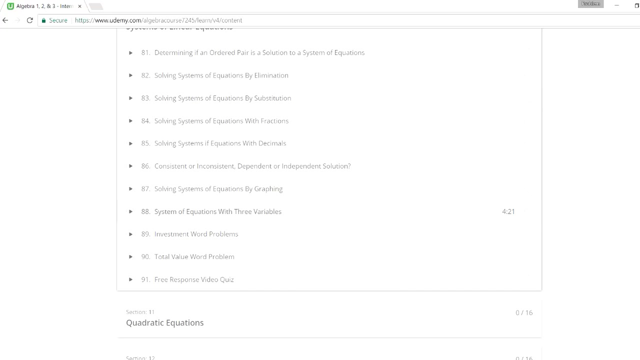 And that's a, A long section. And then factoring You- just That's another topic you need to master- And then system of equations: You can solve it by elimination, substitution. There's also word problems as well. Sometimes you gotta solve equations with three variables.